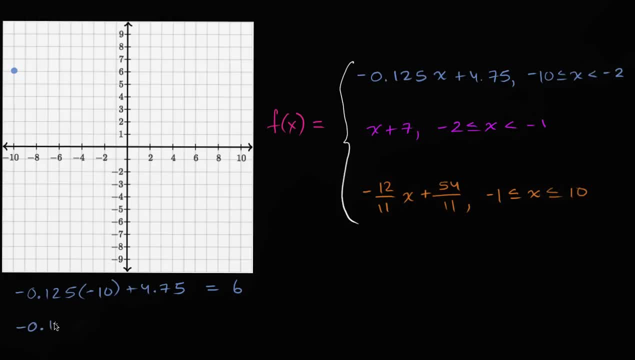 So when x is equal to negative 2, we have negative 0.125 times negative. 2 plus 4.75 is equal to see negative times. negative is positive 2 times. this is going to be point is going to be positive 0.25 plus 4.75.. 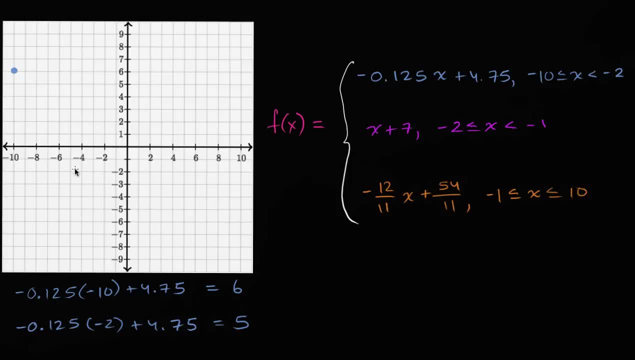 It's going to be equal to positive 5.. Now we might be tempted. we might be tempted to just circle in this dot over here. but remember this interval does not include negative 2.. It's up to and including. it's up to negative 2, not including. 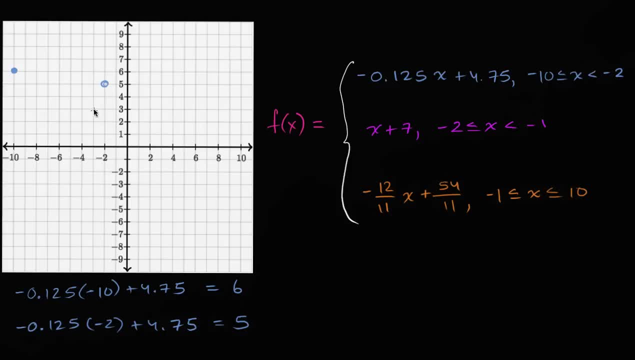 So I'm going to put a, I'm going to put a little open circle there, and then I'm going to draw the line, And then I'm going to draw and I'm going to draw the line. I am going to draw my best attempt. 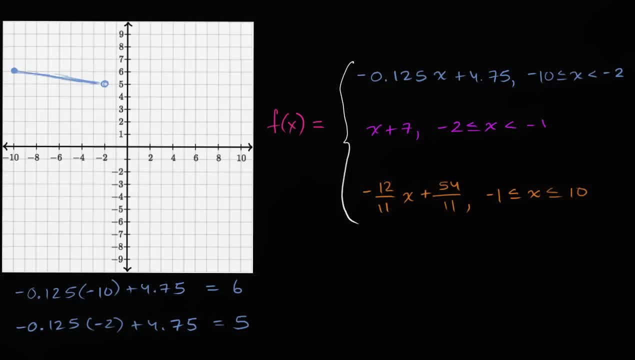 my best attempt at the line. Now let's do the next interval. The next interval and this one's a lot more straightforward. We start at x equals negative 2.. When x equals negative 2, negative 2 plus 7 is. 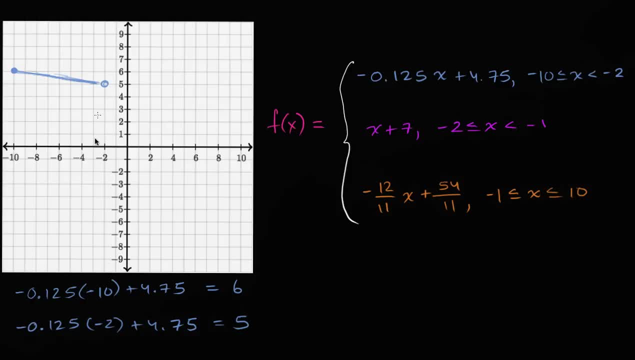 negative 2 plus 7 is 5.. So negative 2, so negative 2 comma 5, so it actually includes that point right over there, so we're actually able to fill it in. And then when x is negative 1,. 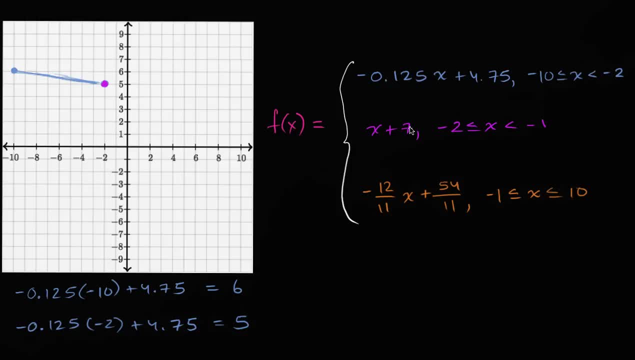 negative 1 plus 7 is going to be positive 7, 6, positive, 6.. But we're not including. x equals negative 1, up to and including. So it's going to be. it's going to be right over here. 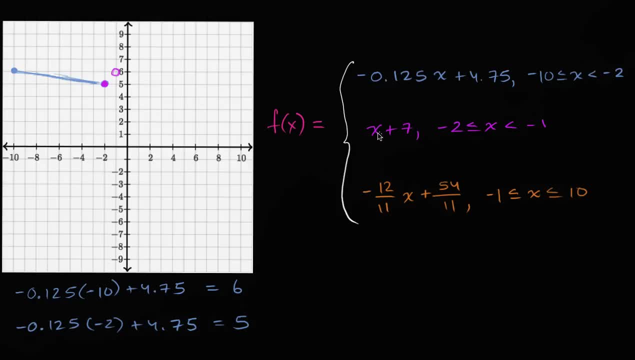 When x is negative 1, we are approaching, or as x approaches negative 1, we're approaching negative 1 plus 7 is 6.. So that's that interval right over there. And now let's look at this last interval. 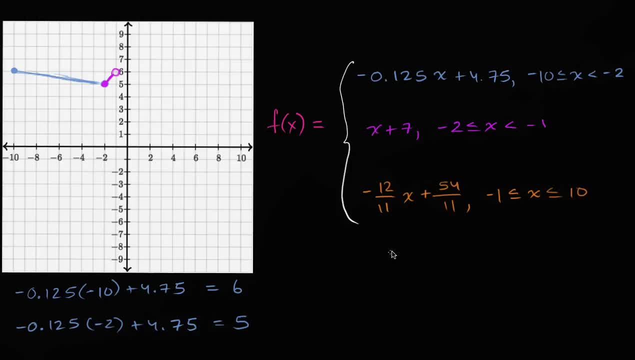 This last interval, when x is negative 1, you're going to have- well, this is just going to be positive- 12 over 11, because we're multiplying it by negative 1, plus 54 over 11,, which is equal to 66 over 11,. 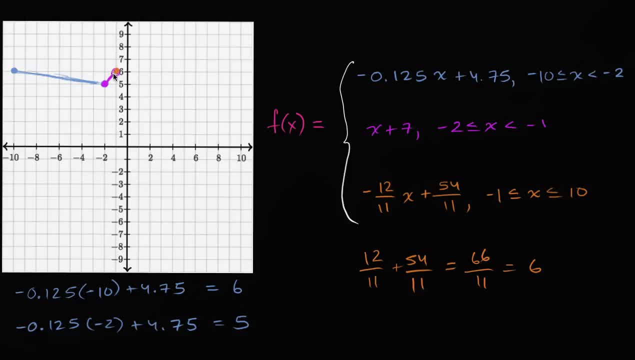 which is equal to positive 6. So we're able to fill in that right over there. And then, when x is equal to 10, you have negative 120 over 11, I just multiplied this times 10,. 12 times 10 is 120,. 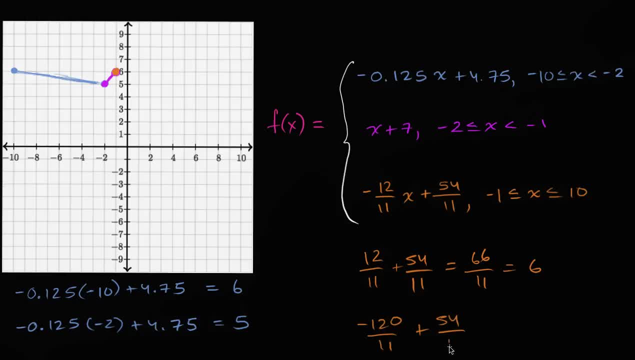 and we have the negative plus 54 over 11.. So this is the same thing. this is going to be. what is this? This is negative 66 over 11, is that right? Let's see if you yeah. 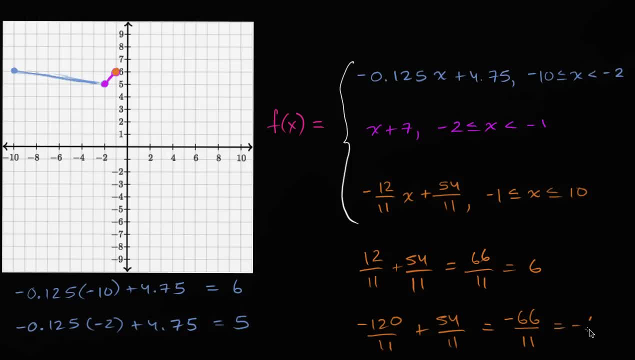 that is negative 66 over 11,, which is equal to negative 6.. So when x is equal to 10,, our function is equal to negative 6. And so this one actually doesn't have any jumps in it. it could have. 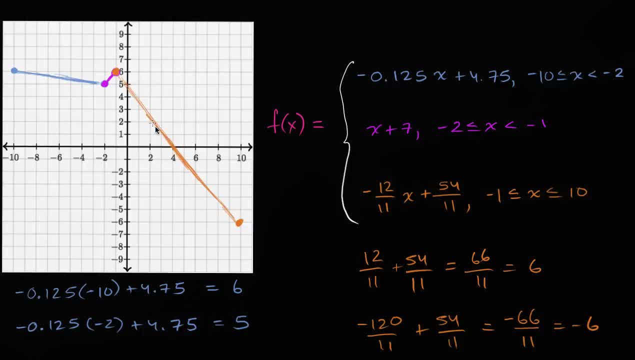 but we see. so there we have it. We have graphed this function that has been defined in a piecewise way. 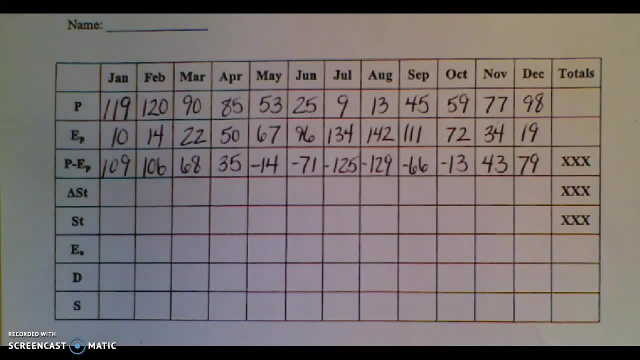 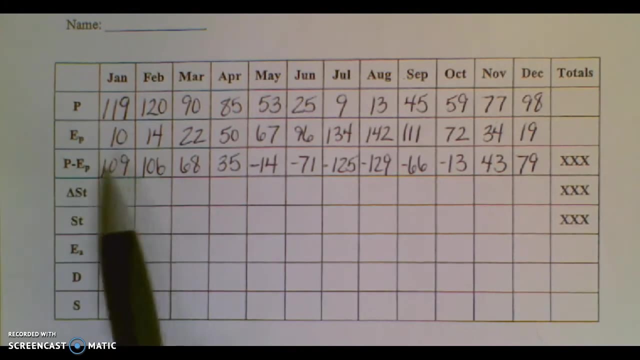 Okay, I'm going to walk you through another water budget here. Just some random city. You can see I've already filled in the precipitation, the potential evaporation and the difference between the precipitation and potential evaporation. Now remember why we're doing this. If you take a look at the precipitation for the month of January, you'll see that it's relatively high compared to the potential evaporation. Therefore, I have a very large positive number. 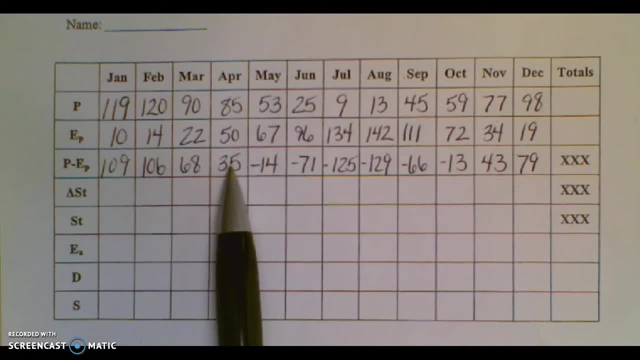 And you can see these positive numbers continue through the first part of the year and don't become negative until May. Why is that significant? What does it mean when these numbers in this third row here become negative? Well, that just tells you that your precipitation has fallen below your potential evaporation. It's a relatively dry month, or a series of months in here. Now, that doesn't necessarily mean you're going to end up with a deficit, because you can tap into your store. 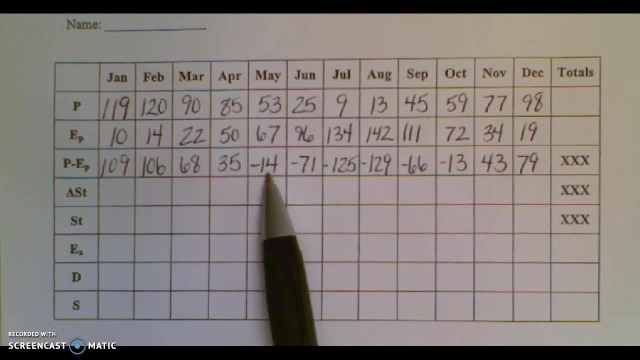 Now I've been thinking about the situation at home a little while now that I'm saving money and taking a shower, but I do want to know what this is going to be like and where this person is saving money. Now it's reduced by coming to January Again. it's just a long, long process. Why? Let me tell you what the transition position look like. 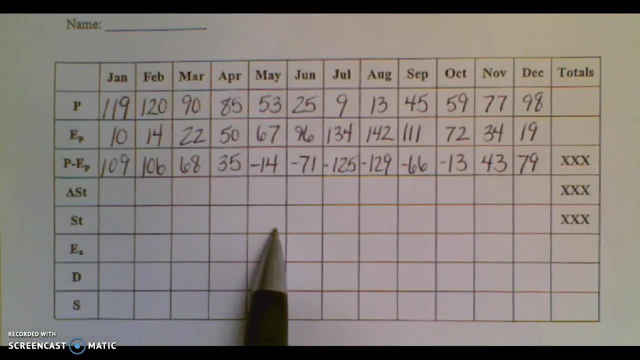 Yourados fund gets an increase in settlement up to a few million. Let's Put that on. So let's turn this one in And look at my graph here. So the permanent deposit e vorbere capital is target. So access payday and credit day.